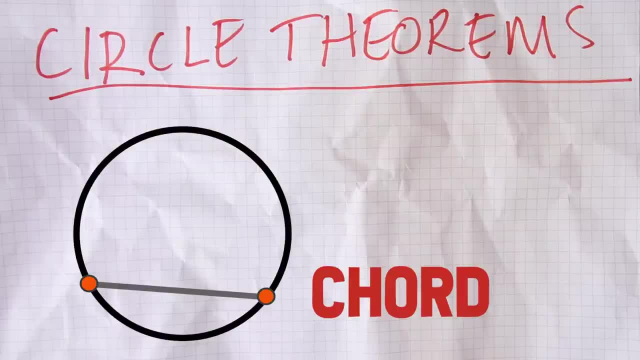 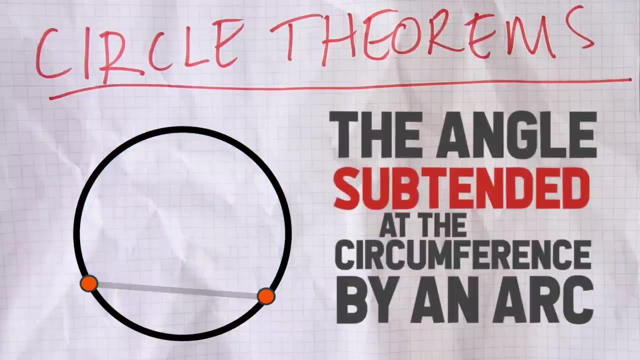 So a chord is just a line between two points on the circumference of the circle And that chord splits the circle into two and we call each of those parts segments. The final piece of language is a phrase using this word subtend. If we go back to our points on the circumference, 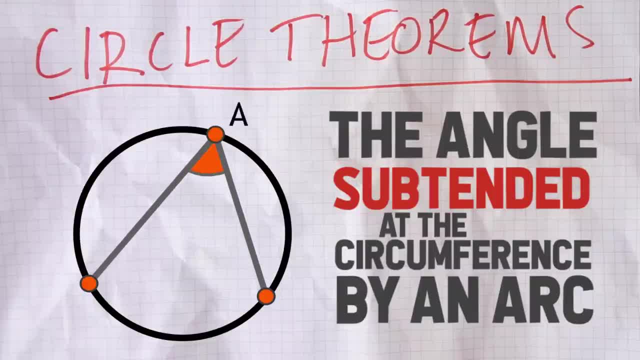 of the circle and we take a line from each of them to create this angle on the circumference at point A. we could describe that as the angle subtended at the circumference by an arc. What does that mean? Well, subtend just means the angle created at a particular point. In this case, the particular point is on the 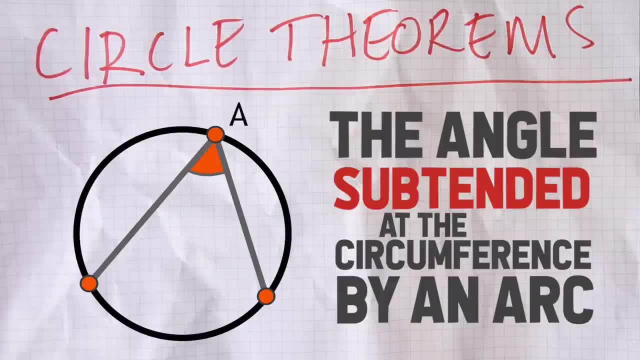 circumference of the circle. So subtended at the circumference just means the angle that we've created on the circumference of the circle, And the last part about an arc just tells us that the angle was created by taking two lines from each end of an arc. If we put that all together then the whole thing means the angle created. 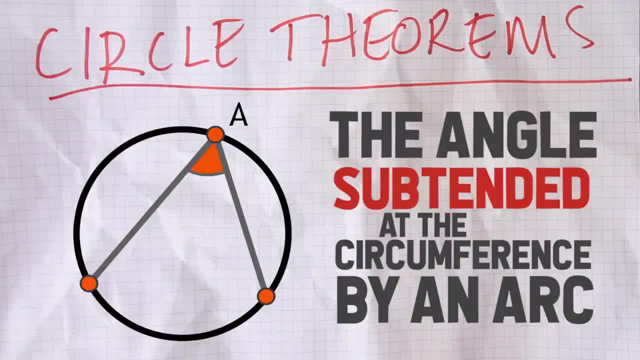 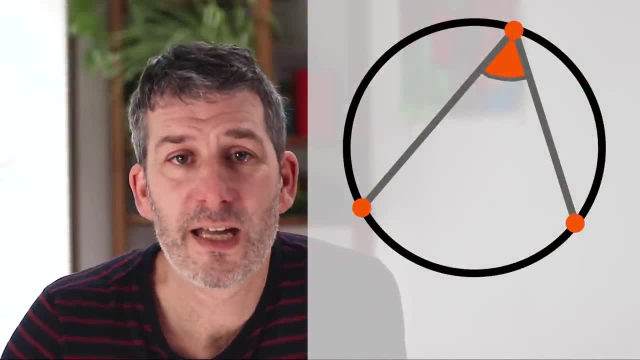 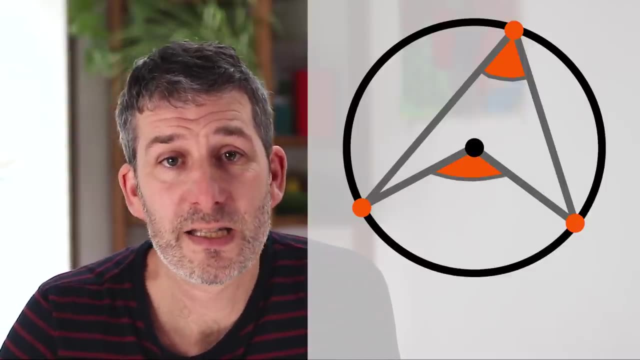 on the circumference of the circle by two lines coming from either end of an arc. right, The angle subtended by an arc. If we create an angle at the center of the circle coming from those same two points, in other words, an angle subtended at the. 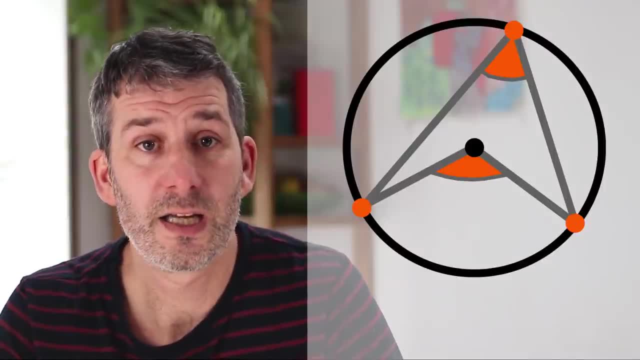 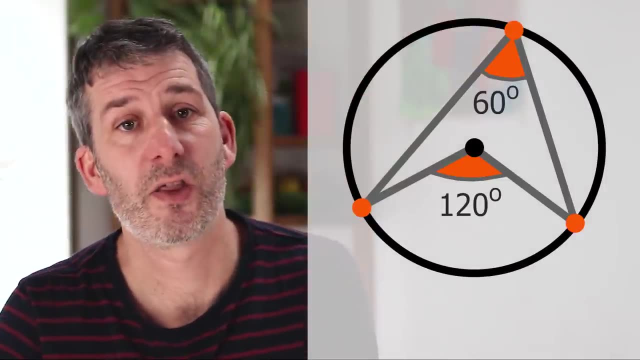 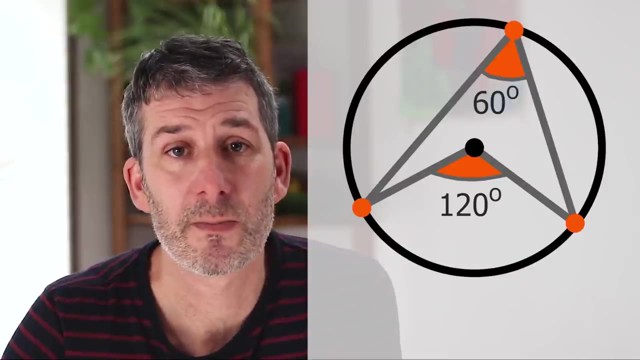 center of the circle by the same arc, then the angle created at the center will always be double the one at the circumference, Always. Okay, that's our first theorem. The angle subtended by an arc at the center is twice the angle subtended at the circumference. 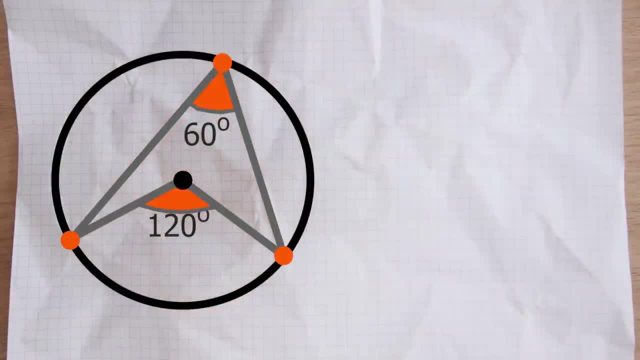 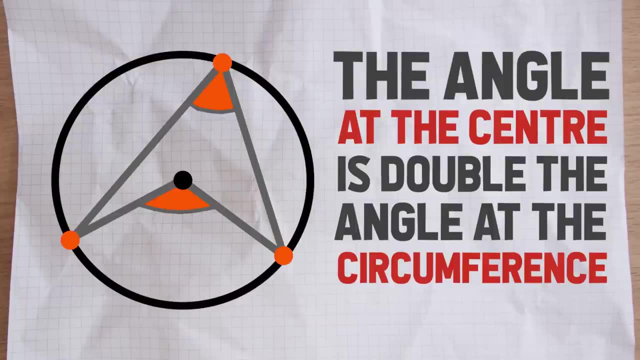 That's quite a mouthful to remember. so we can simplify it to: the angle at the center is double the angle at the circumference, And that is always the case. Even if we move this point around, it will always be the case. So just be aware that it may well look very. 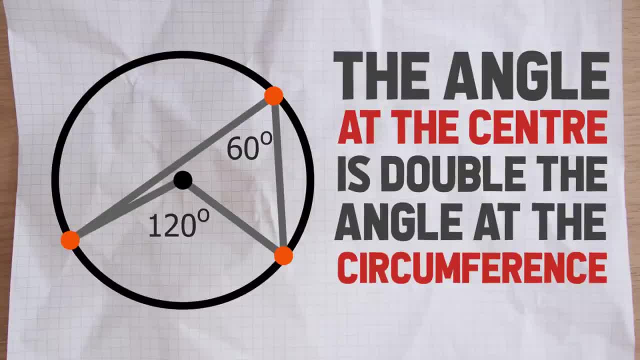 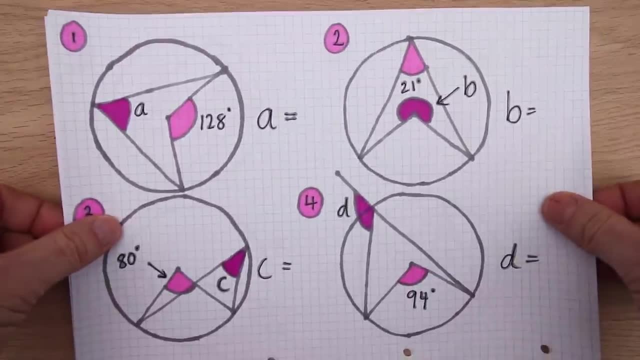 different, Sometimes like this arrow shaped example, or at other times it could look like this, which actually looks completely different, But in both cases the angle at the center is always double the angle at the circumference. Here are three questions. then Pause the video. 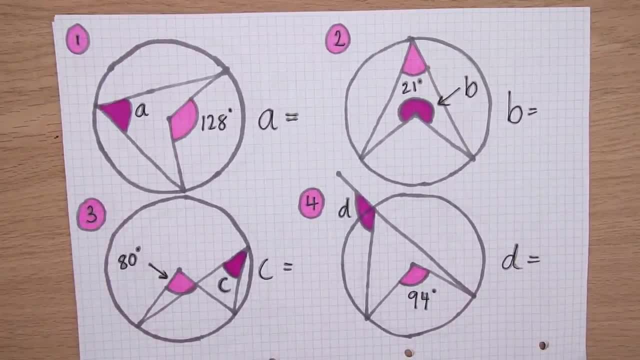 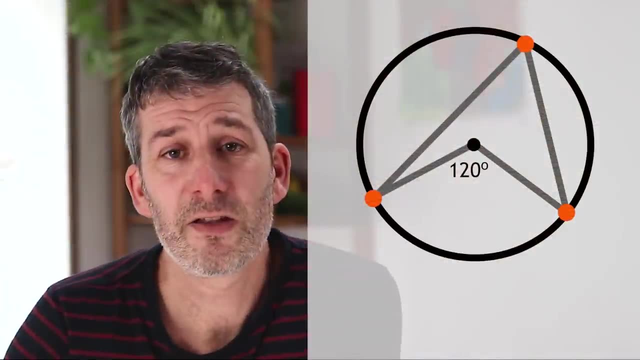 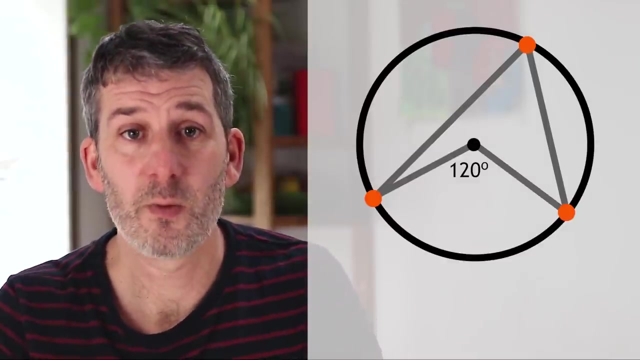 find the missing angles and I'll show the answers in a moment. The second theorem we'll look at follows on from the first one. We just established that it doesn't matter where that angle on the circumference is. it will always be half of the angle at the center, And you can see as I move the point around. 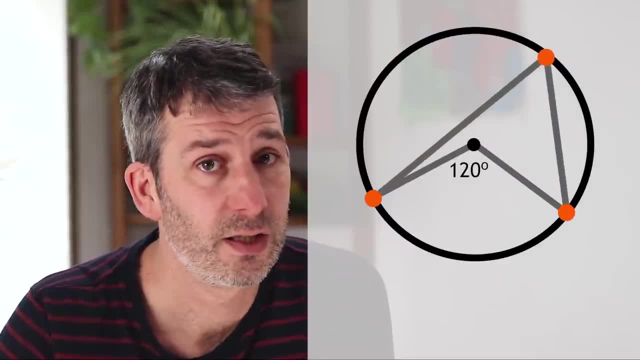 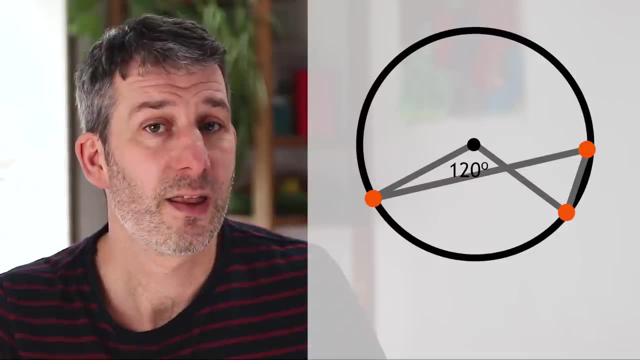 the circumference, the angle at the center isn't changing And therefore, if the angle at the center is always twice the angle at the circumference, it must follow that the angle at the circumference isn't changing either. Just for clarity, if we show that, 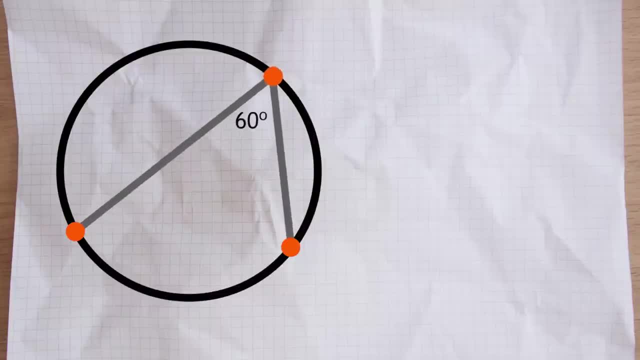 without the angle at the center. you can see that the angle at the circumference never changes. That is as long as it stays in the same segment, In other words on the same side of those two points. As soon as you move that angle down below the two points into, 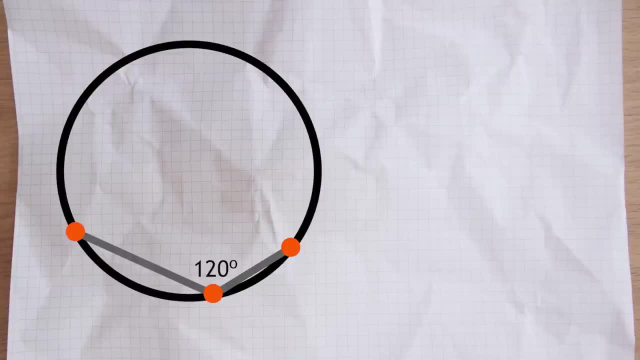 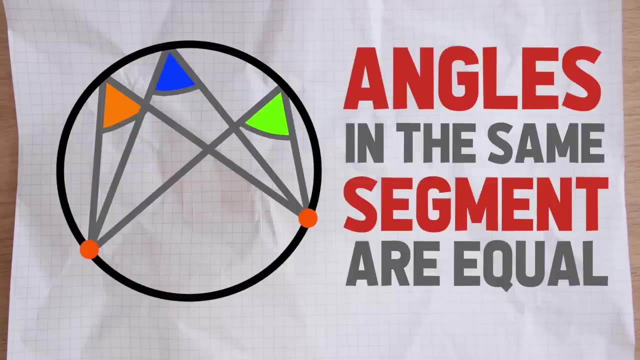 the other segment, it changes. We say angles subtended by an arc in the same segment are equal, or put more simply, angles in the same segment are equal. All of these angles will be equal to each other. Pause the video, then have a go at these questions and I'll be back with the answers. 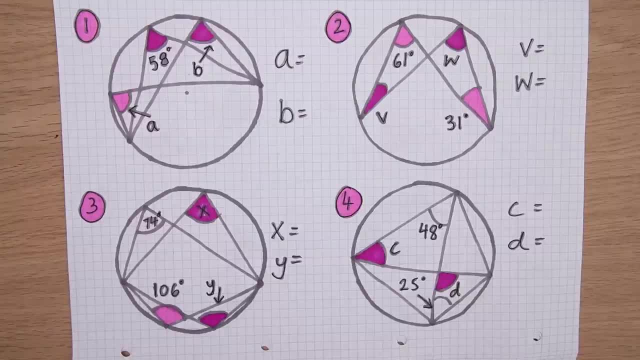 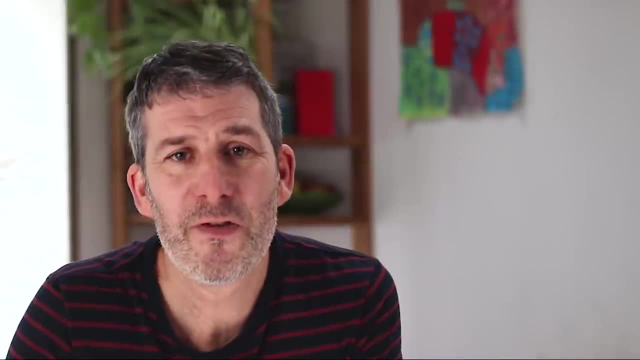 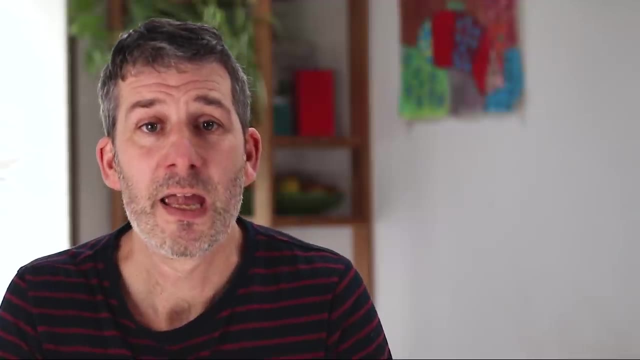 in a few seconds. By the way, if you found this video useful, it really helps the channel to grow if you subscribe or give the video a thumbs up or share it with your friends. Thank you very much. if you've already done one of those things Also, don't forget to have a look at my 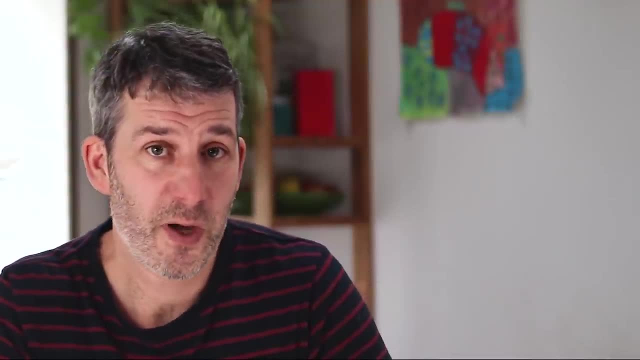 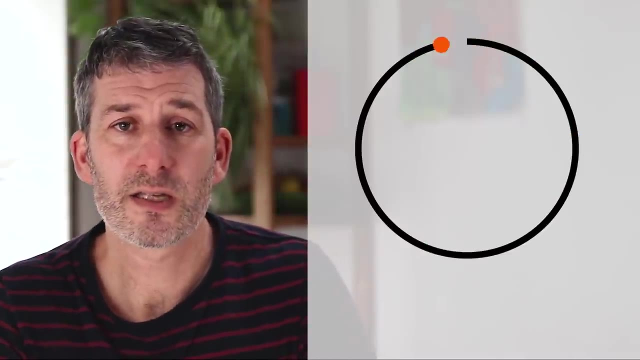 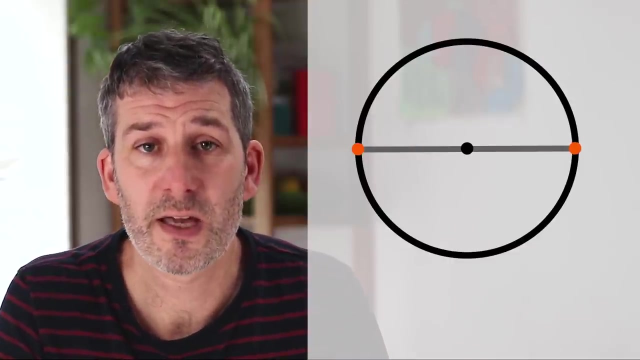 Facebook page That's just Maths Kitchen as well, and I post additional things up there. Back to the circles. then If we draw a line passing through the center of the circle, we call that the diameter. Now, if we focus on just half of that circle, a semicircle- 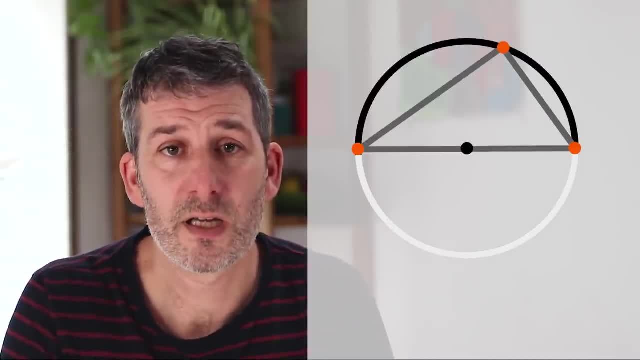 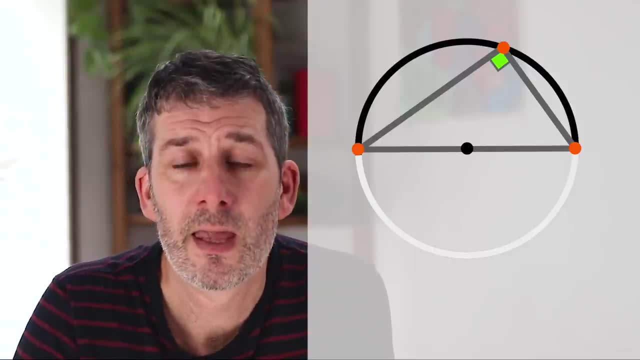 in other words, and create an angle from either end of that diameter to somewhere else on the circumference, that angle will always be a right angle- 90 degrees- And because of the second theorem we looked at, we know that if it's a right angle here, 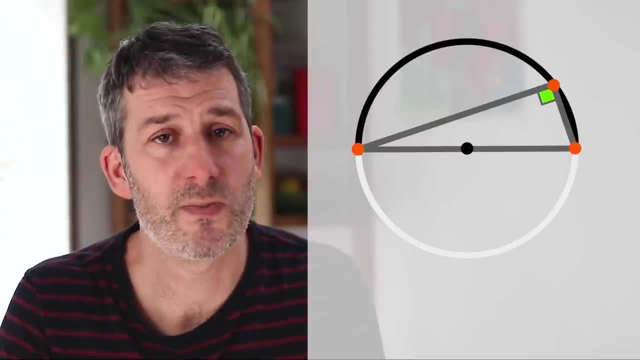 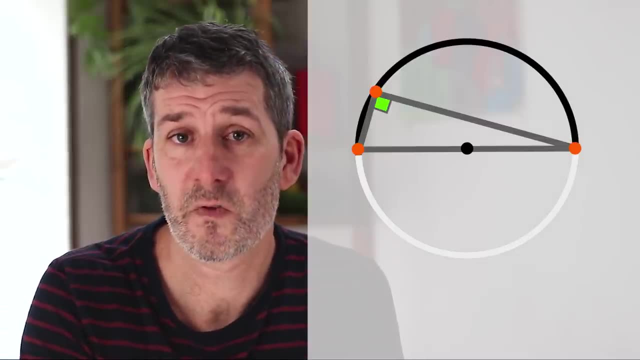 if we move that point around the circumference, it won't change. It will always be a right angle. And in fact that links to the first theorem as well, because the angle at the circumference- in this case 90 degrees, we know- is always half the angle at the center, And that's true. 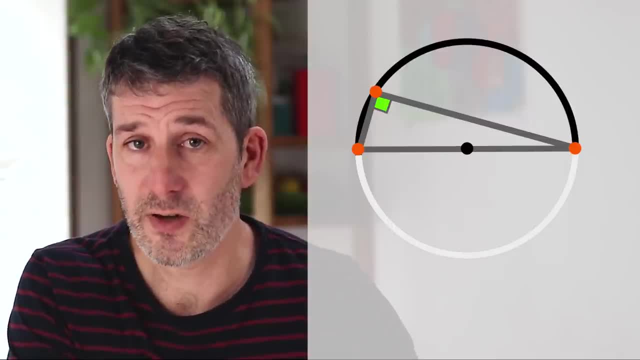 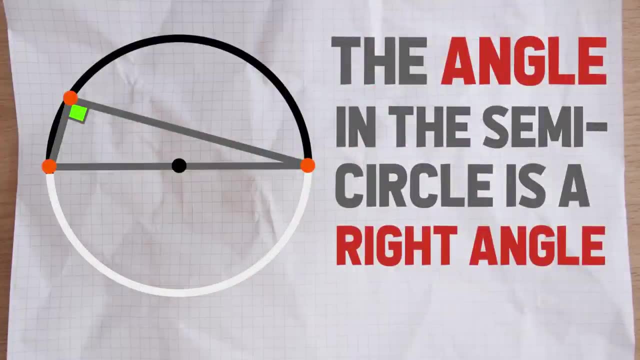 here as well, isn't it? Because the angle at the center is 180 degrees. It's just that straight line. So 90 is a half of 180 degrees. So that's the third theorem. The angle in a semicircle is a right angle. Pause the video. 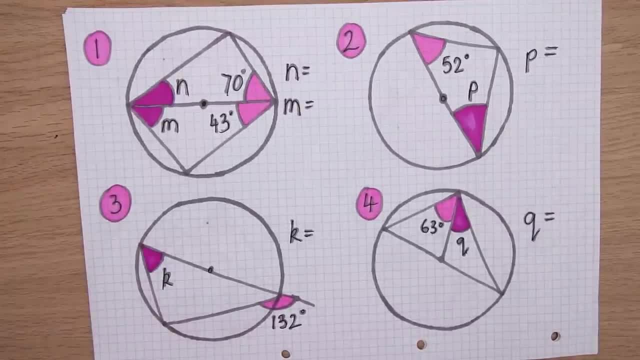 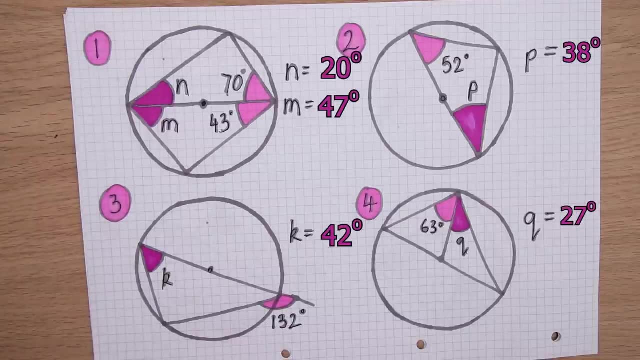 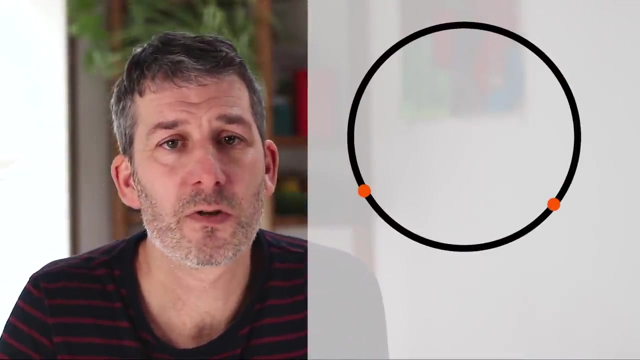 have a go at the questions and I'll show the answers in a moment. Theorem number four: then You can see on the diagram here a four-sided shape, a quadrilateral. You can also see that each vertex or corner is touching the circle. 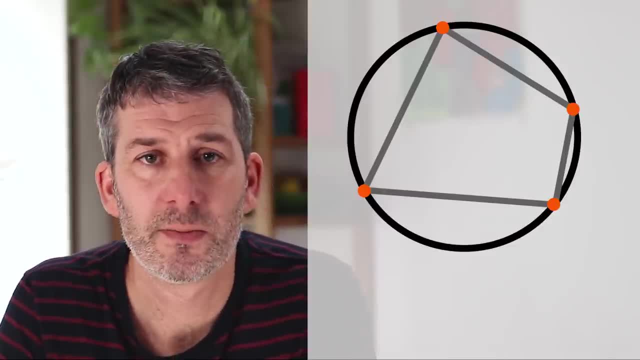 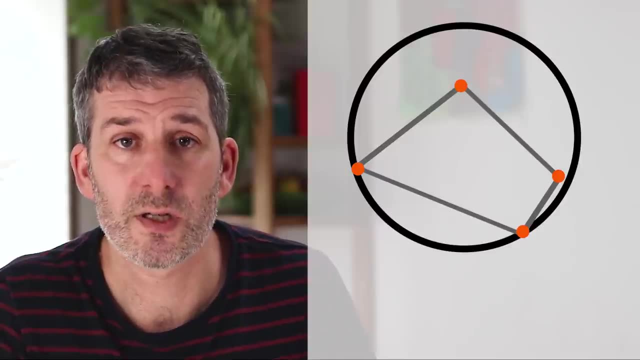 That makes it what we call a cyclic quadrilateral. This example is also a quadrilateral, but you can see that not all of its vertices are touching the circle, so it's not a cyclic quadrilateral. Cyclic quadrilaterals, then, they must have all the vertices touching the circumference. 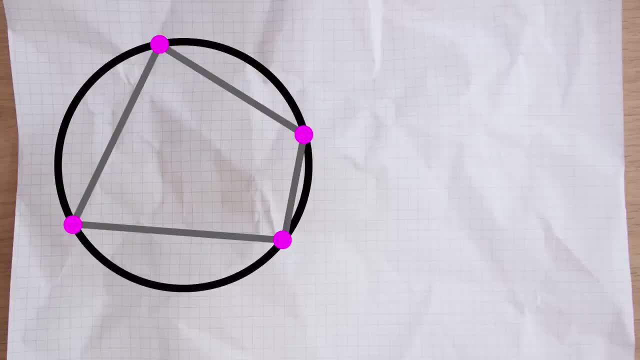 of the circle, And the rule here is that the opposite angles will always add up to 180 degrees. So if this angle is 80 degrees, then this other one must be 100 degrees. If this angle is 65 degrees, this other one must be 115, so that they add to 180 degrees. 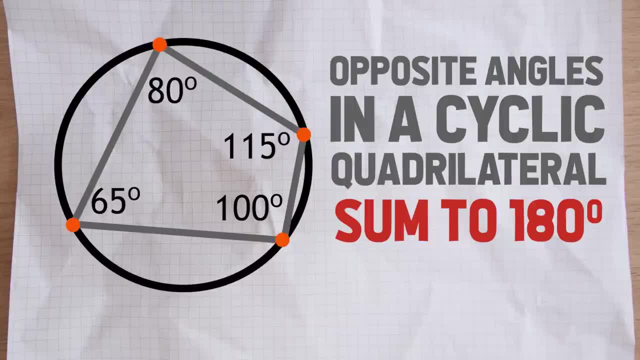 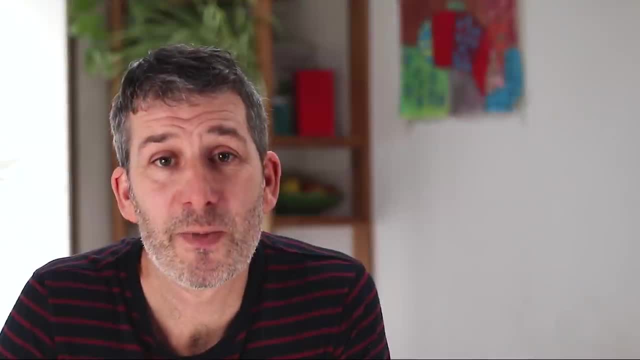 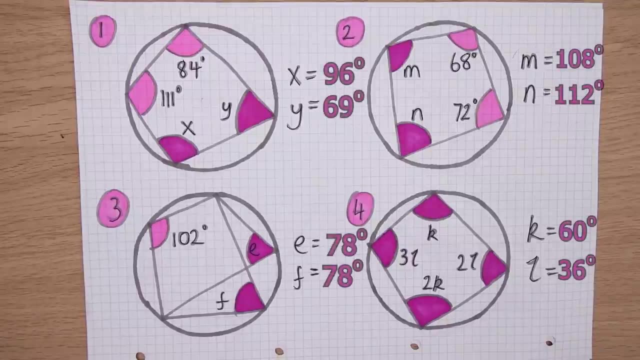 That's our fourth theorem. then Opposite angles in a cyclic quadrilateral sum to 180 degrees. Pause the video, have a go at the questions and I'll be back in just a moment. Now we need to talk about tangents. 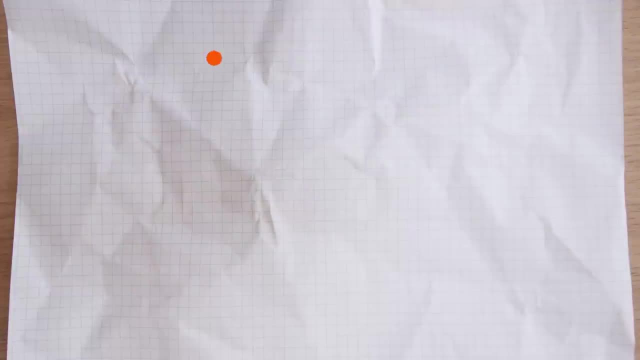 First of all, what are tangents? Well, a tangent is a line that just touches the circumference. It doesn't go into the circle, it just touches that circumference. And there are three theorems that involve tangents. The first is that if you take a line from the centre of the circle to meet the tangent, 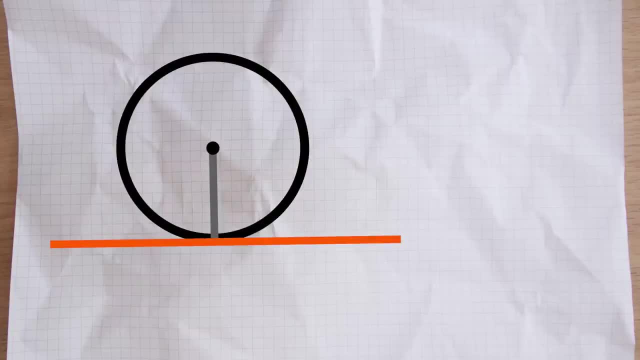 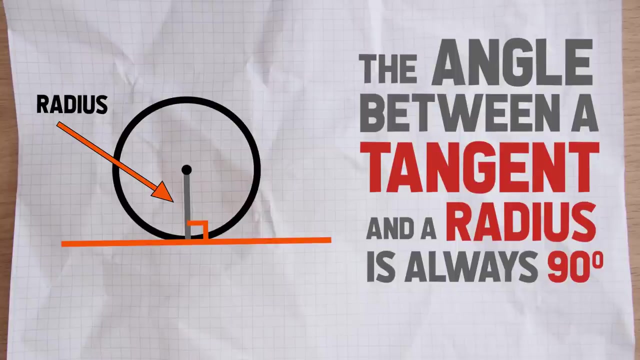 at the circumference. it will always meet at a right angle, That line from the centre of the circle to the circumference. we just call that the radius, or radii if you're talking about more than one of them. So the rule is that the angle between a tangent and a radius is always 90 degrees. 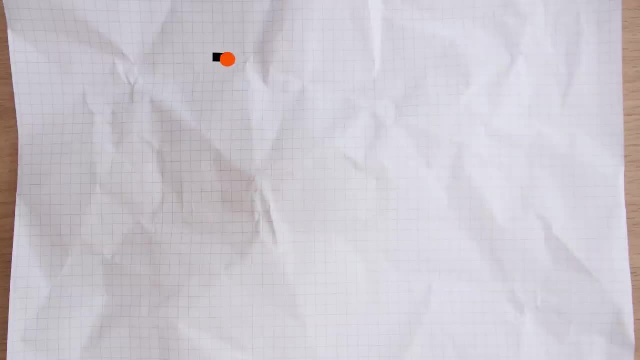 The second theorem to do with tangents is that tangents that meet at a point are equal in length. In other words, if you have two tangents like this meeting at a point- in this case point A, those two lines will always be the same length. 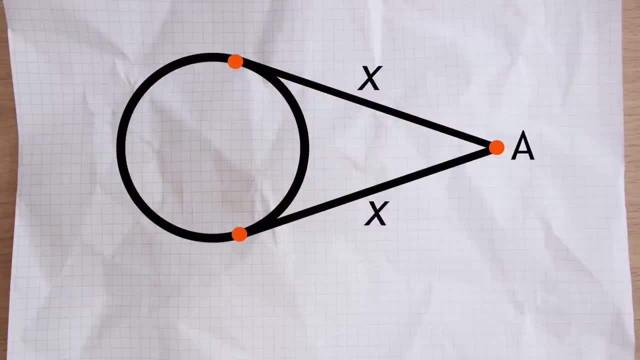 And we can use those two facts to find the missing angles In these kinds of questions. you can see, we have a quadrilateral where two of the sides are in fact tangents to the circle and these other two lines are radii. They go from the centre of the circle to the circumference. 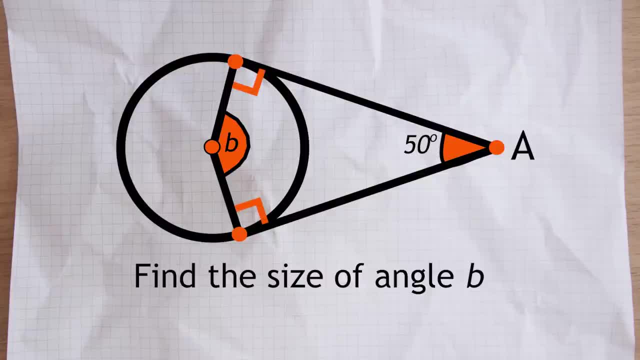 Therefore they form a 90 degree angle where they meet those tangents. So now we know three of the four angles in the quadrilateral, And we also know that angles in a quadrilateral always add to 360 degrees. So if we subtract those three angles from 360 degrees, that will tell us what the missing. 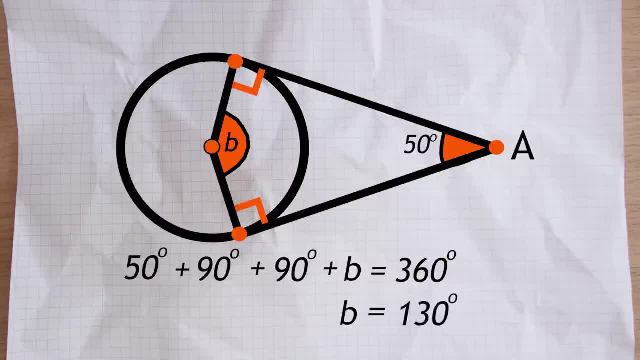 angle is, And in this case it's 130 degrees, And the final theorem to do with tangents is the Alternate Segment Theorem, which is that the angle between a tangent and a chord is equal to the angle in the alternate segment. What on earth does that mean? 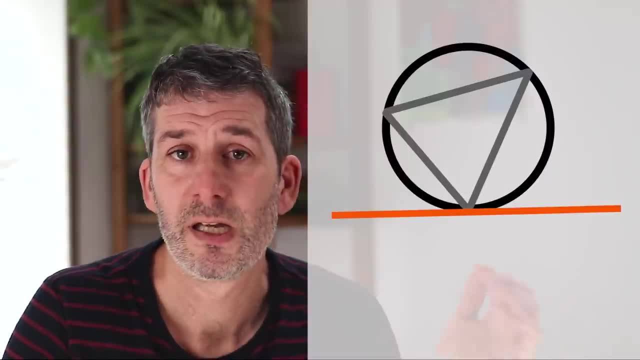 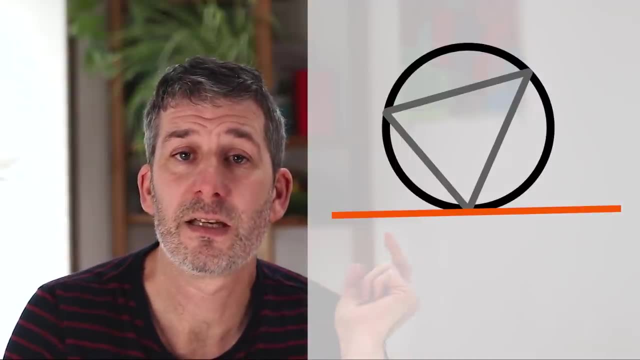 Well, it just means that if you have this kind of situation, the angle created between the chord- Remember that's just a line connection Connecting two points in a circle- And the tangent, the highlighted angle there, is equal to the angle on the other side of. 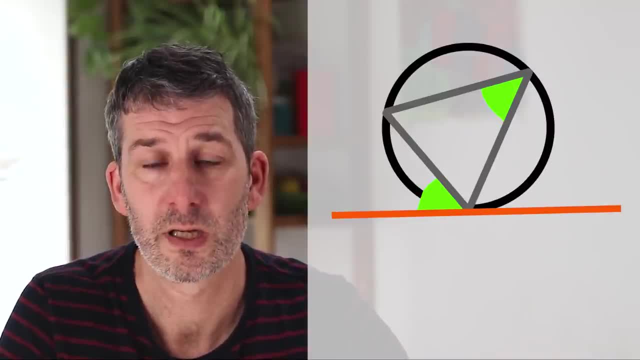 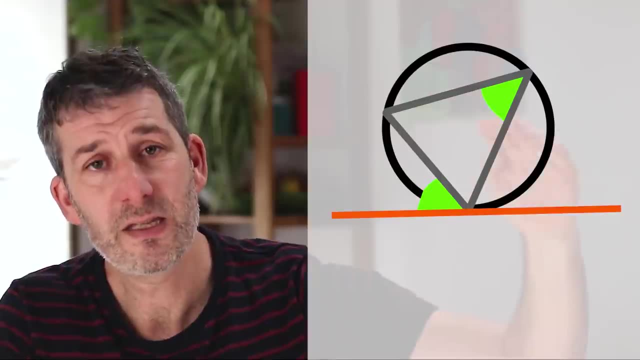 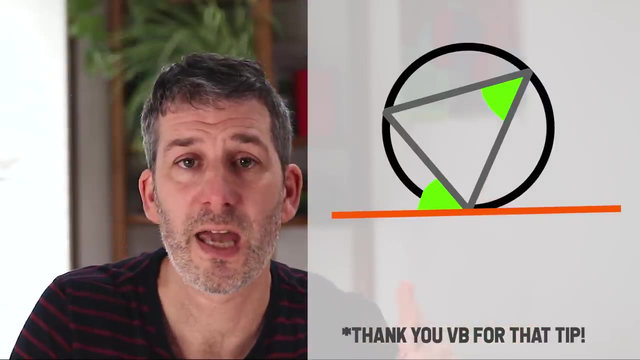 the chord, In other words in the alternate segment. I always found this one really difficult to remember, but I have found it helpful to think of inside, opposite outside. In other words, the angle inside the triangle is equal to the angle that is opposite, and 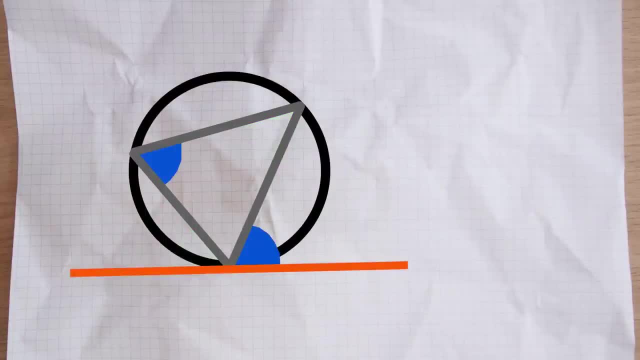 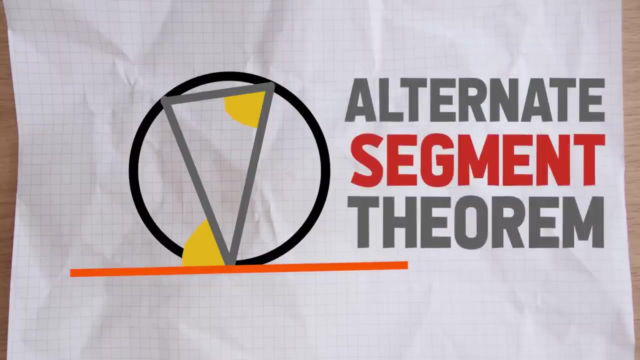 outside Right. so this angle is equal to this one, This angle is equal to this one And this angle is equal to this one Inside, opposite outside. We call that the Alternate Segment Theorem. Pause the video, then see if you can find the missing angles in the following questions. 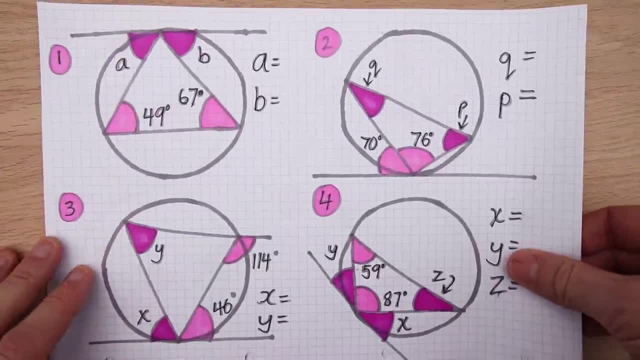 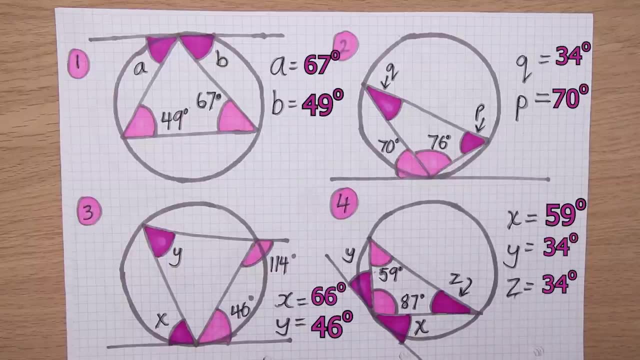 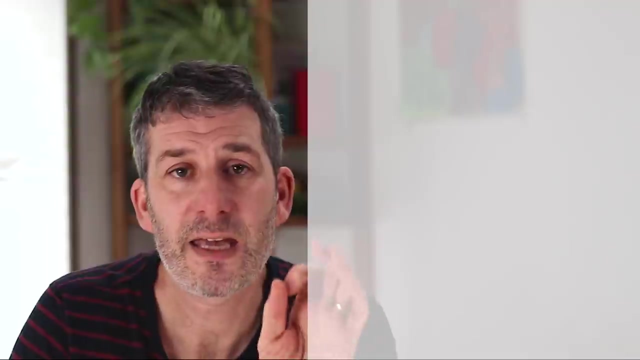 and I'll be back in just a moment. That's all of the theorems out of the way, but there is one thing left to cover, and that is if you have a triangle inside a circle where two of the sides are radii of the circle. 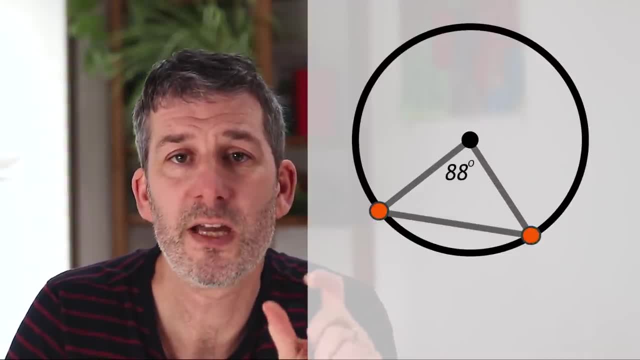 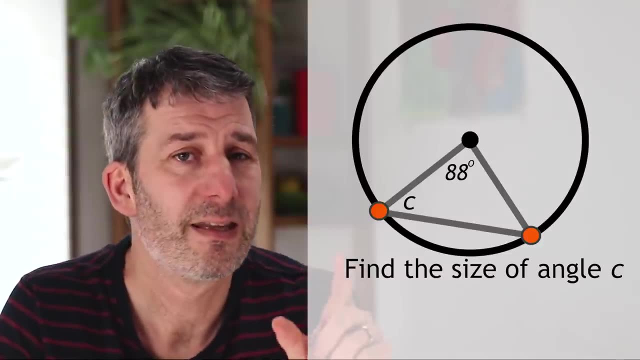 as in this example, If two sides are the radii of a circle, then they must be the same length. So you therefore have an isosceles triangle, And that could be useful to note, because in an isosceles triangle the two points are: 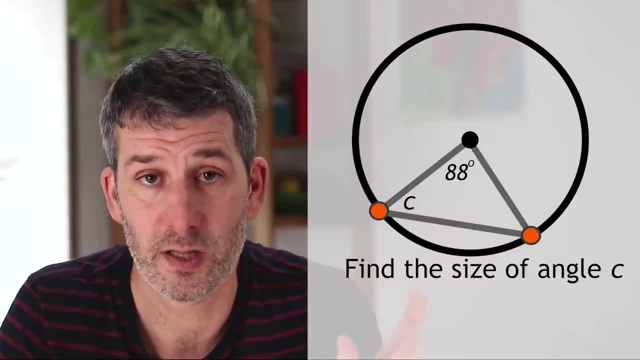 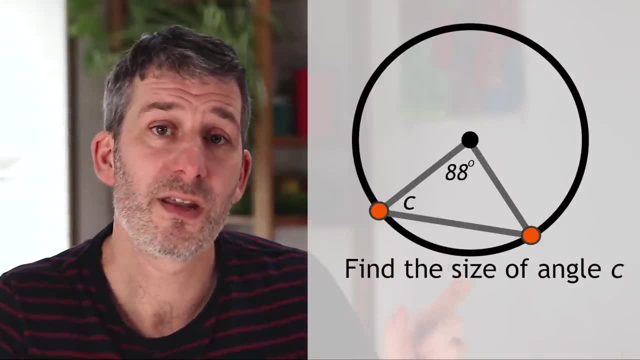 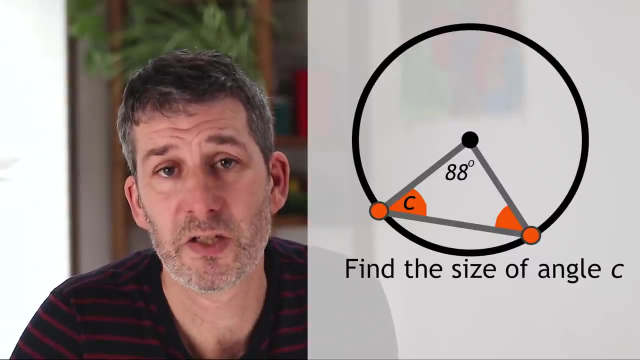 the same length, Right? So in a question like this, we can see that we have an isosceles triangle and therefore we know that these two angles will be equal to each other. We also know that all three angles in that triangle will sum to 180 degrees, and therefore 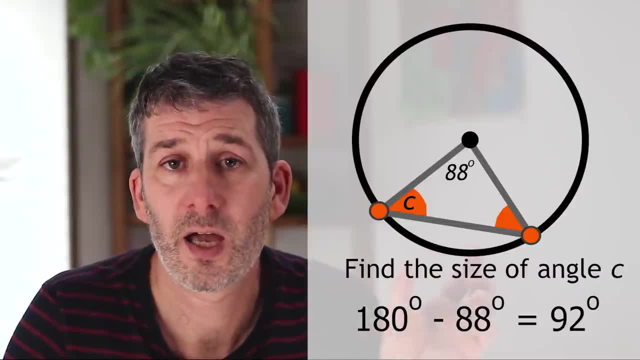 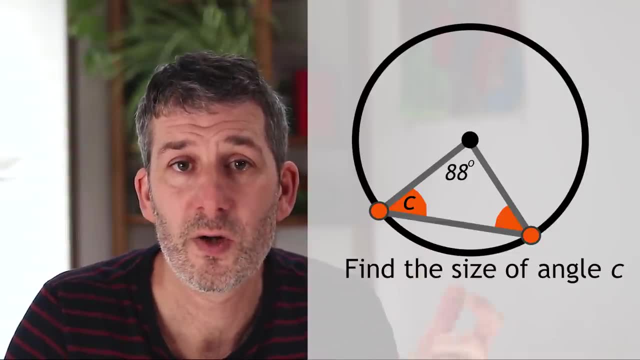 these two missing angles must add to 92 degrees 180 minus 88. And because they're the base angles in that isosceles triangle, we know that they're going to be equal to each other, And so they must be half of 92.. 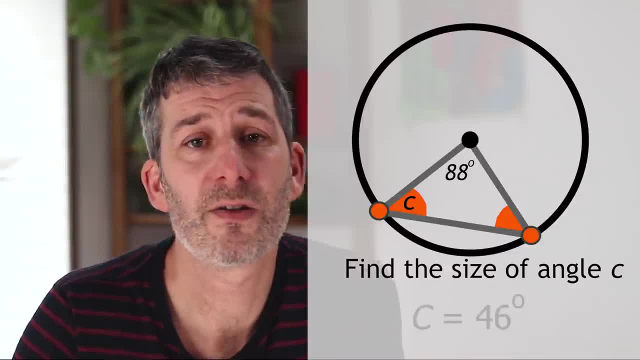 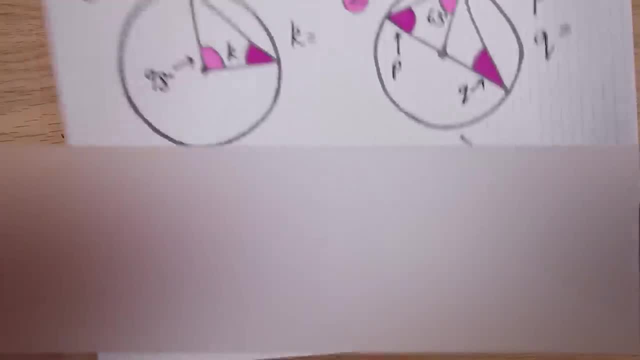 And half of 92 is 46. So our missing angle there is 46 degrees. As ever, here are a few questions for you to practice. I'll be back in a few seconds for my tips on how to solve circle theorem problems in. 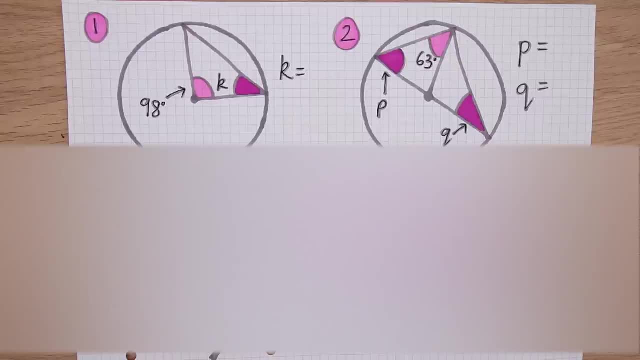 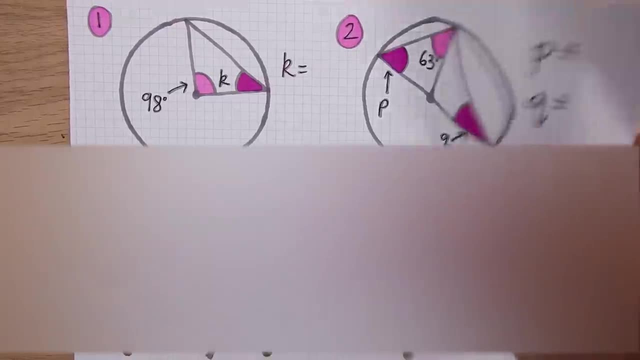 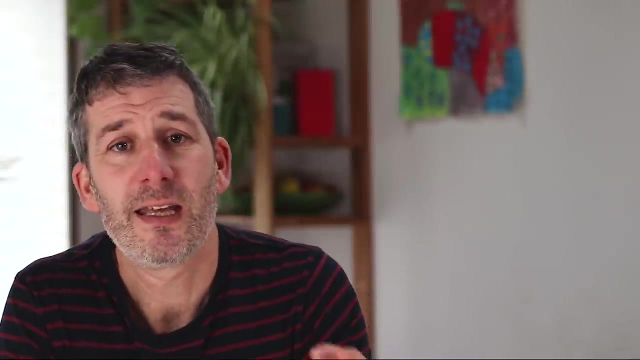 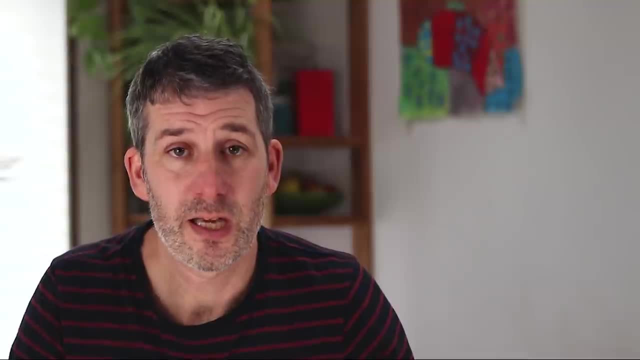 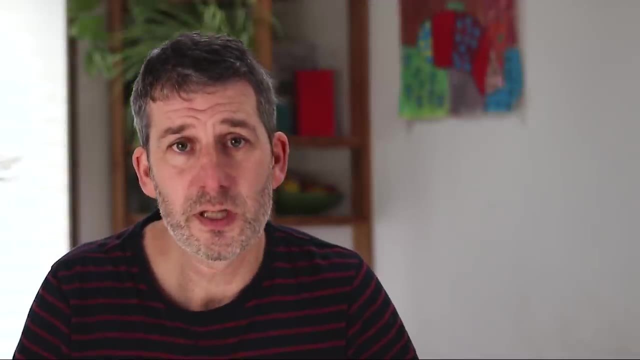 you're trying to find and just ask yourself: are there any missing angles here that I can get? Sometimes just kind of zooming out like that, shifting your focus, can be enough to unlock the problem and just get you moving along. If it doesn't help, then ask yourself if you can recognise any of the possible missing angles.